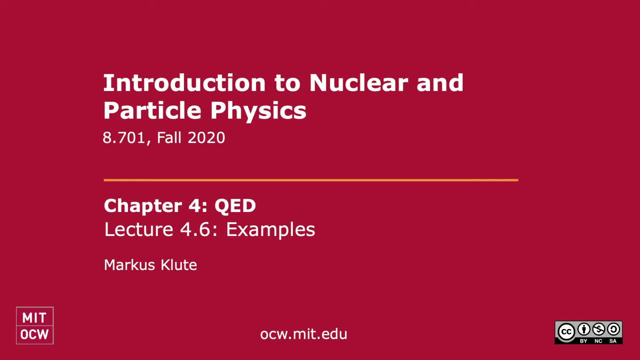 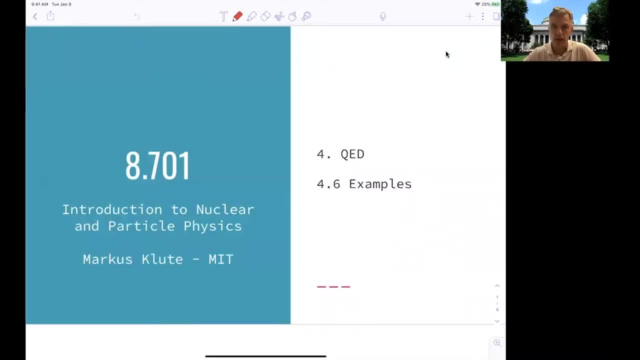 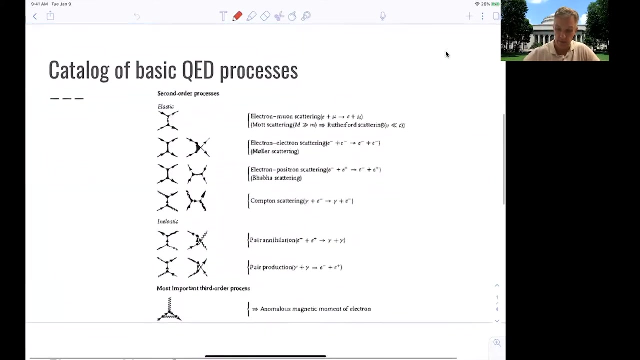 Welcome back to 8.7.01.. So in this lecture we are going to start looking at an example of the process for which we can now, with all the tools we have in hand, calculate the matrix element transition amplitude. All right, In more general terms, we can look at all. 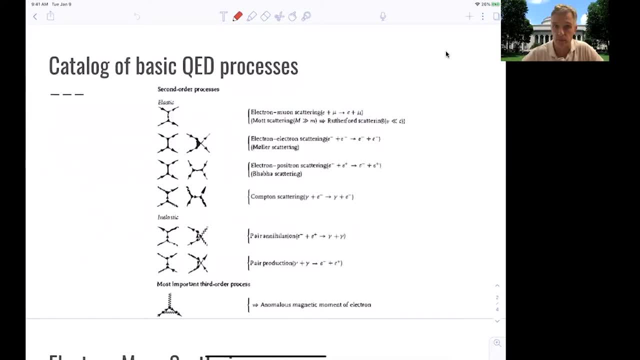 the examples, and they're listed here: second-order processes and one-third-order processes. We are going to discuss them in more detail as we go along. This is really just to give you feedback for the different kinds of processes we're going to look at. So the first one is: 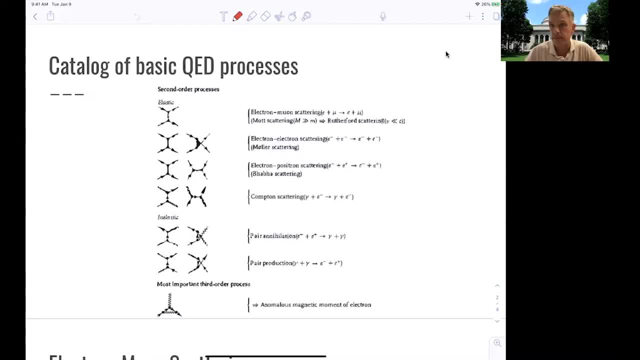 elastic scattering. It's muon-electron scattering. That's the one process we're going to look at in more detail. Why? Because this is the simplest case For this process. there's only one leading-order diagram, which is exactly the same as the first one, So we're going to look at the first one. 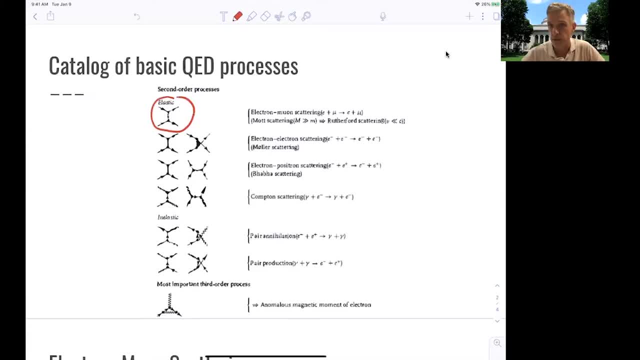 So we're going to look at the first one. So we're going to look at the first one. For other processes where we have the same particle interacting, we find that we do have to consider multiple diagrams, For example this one: here We have electron on electron. 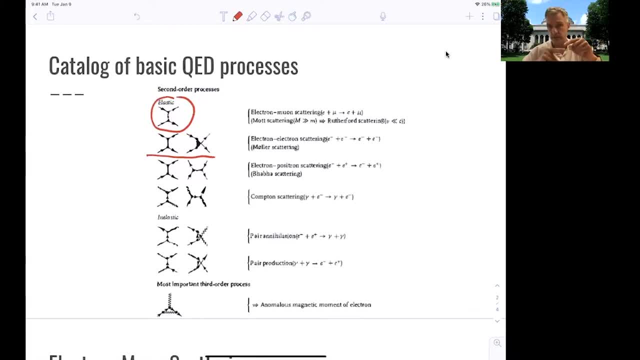 scattering, And so we have to calculate not just this leading diagram, which looks exactly like the one for the muons scattering, but we also have to include the cross-term term where we change the outgoing electron lag, and so on. The processes are including electron positron scattering, which is called Barber. 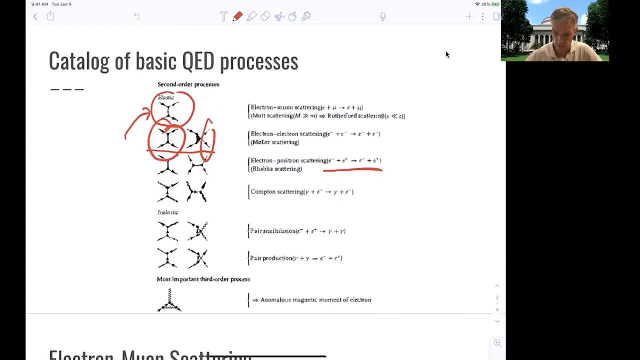 scattering- Compton scattering, which we discussed the kinematics for already, but also inelastic processes like pair emulation or pair production. There's a very interesting diagram here which is a third-order diagram, which is responsible for the anomalous magnetic moment. We'll talk more about that when we talk about higher order correction. 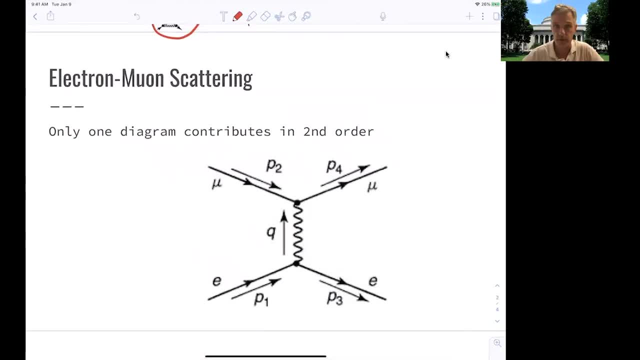 So let's have a look at this electron-muon scattering process. So only one diagram contributes at second order, and so you have an electron and a muon scattering via the exchange of a photon. This is, after all, a QV diagram. So now, how do we calculate the magnetic moment?